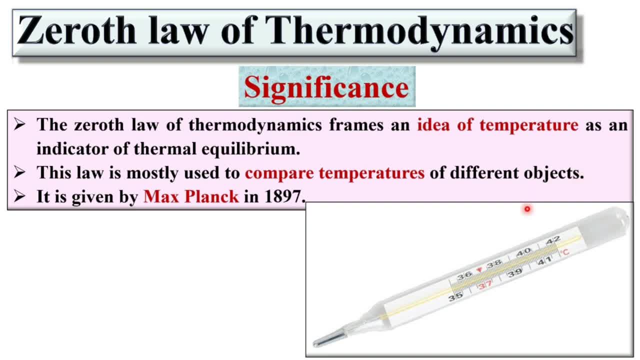 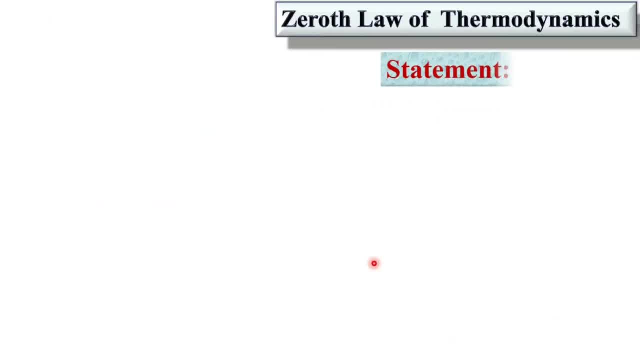 temperatures of different objects. It is given by Max Planck in 1897.. Now see the statement of the zeroth law of thermodynamics If two bodies, A and B, are in thermal equilibrium with third body C. So this is the condition of the statement of zeroth law of thermodynamics. 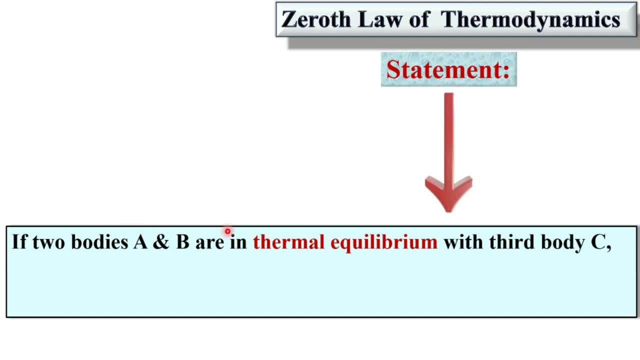 So let me draw over here the condition of the statement. So here two bodies, A and B, are in thermal equilibrium with third body C. So this is the body A and body B, and both are in thermal equilibrium with the third body C. So I am going to show over here: body A is in thermal equilibrium. 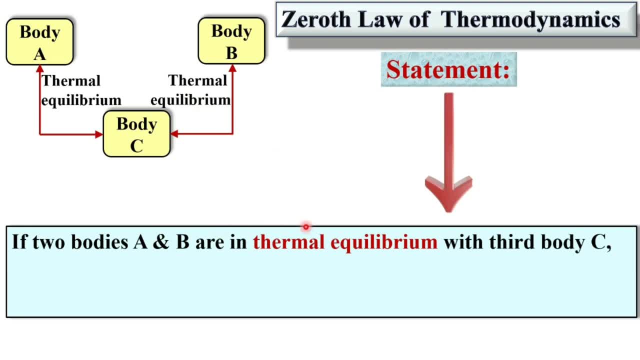 and body B is in thermal equilibrium with body C. So this is the condition of the statement. Now next, the two bodies, A and B, are also in thermal equilibrium With each other. So I can say both body A and body b are in a thermal equilibrium. 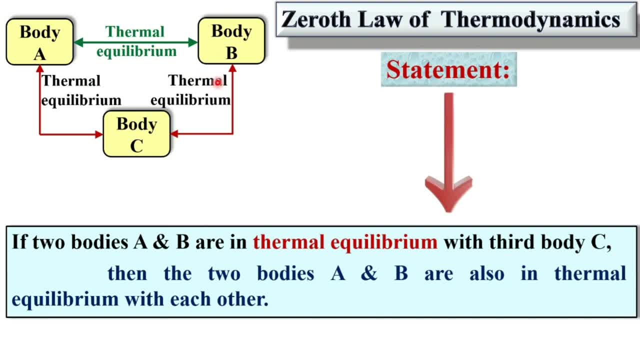 two part. first is the condition: if the two body, A and B, are in thermal equilibrium with body C, then the two bodies A and B are also in thermal equilibrium. So this is the statement of zeroth lobe thermodynamics. Now see what is exactly the meaning of thermal equilibrium. 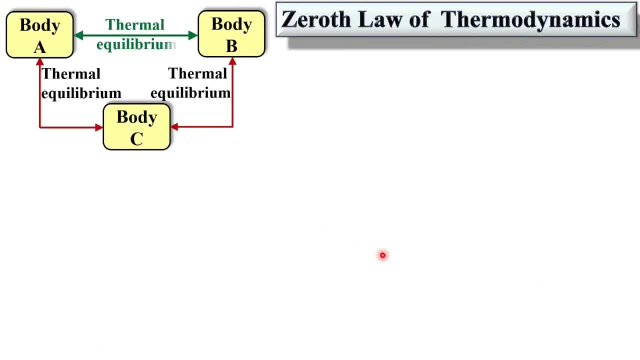 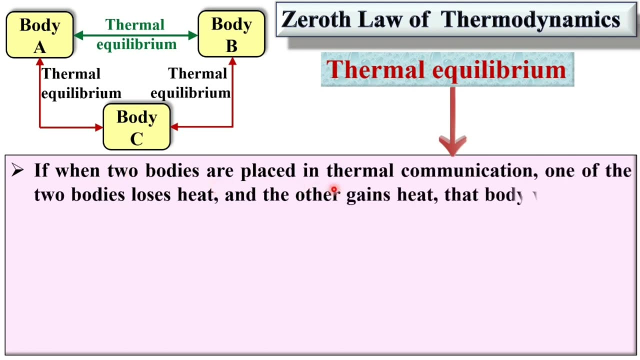 So already we have discussed this is the graphical representation of the zeroth lobe, thermodynamics. Now the meaning of thermal equilibrium: if, when two bodies are placed in thermal communication, one of the two bodies losses heat and the other gains heat, 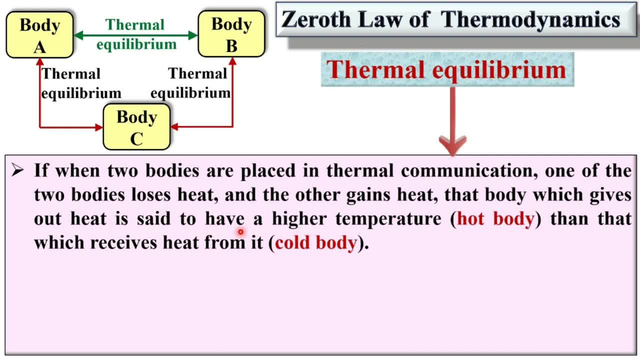 That body which gains heat will lose heat. So this is the representation of the zero lobe thermodynamics. So already we have discussed this is the graphical representation of the zeroth lobe gives out heat, is said to a higher temperature means hot body, then that.